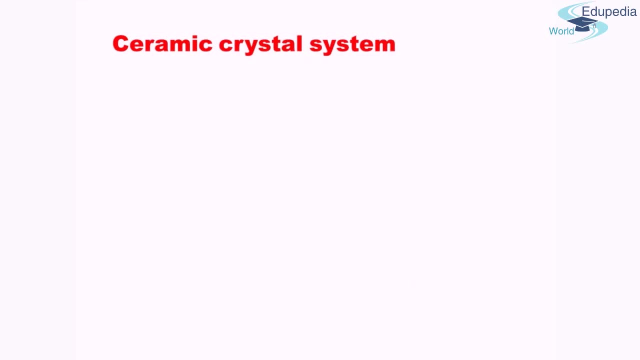 Okay, so to begin with let us see the fundamentals about ceramic crystal system. As I said, that for a ceramic crystal system there have to be at least two different types of atom. right, because one type of atom means it is a element and it will fall under one. 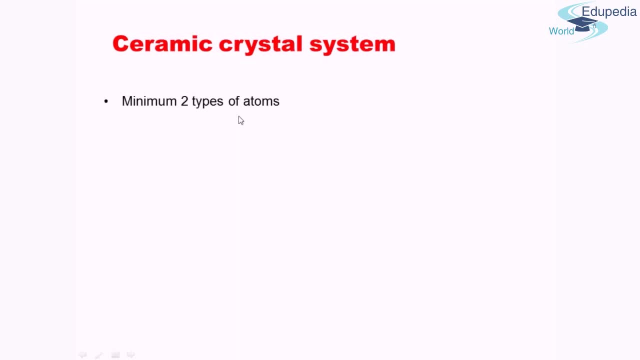 of the fourteen Bravais lattices right, So they need to be two type of atoms for allowed ceramic to exist. Now, the two types of atoms. within our discussion for the time being, considering there are just two different types of atoms. Not more than two. So, given there are two different kinds of atoms, There are two types of ceramic events, one body and other just to join topos. but especially the last point is the power of two concepts. An atom can power the each other. If you have of two certain types of atoms, remember that there are сначала two types of atoms. Similarly, an element with specific atom, for example, is a male and second, one should be faster than the other, Because there are a little bitWould be must laughing. as comprises the difference in the number of p-? firstly, but overall it is different from frames of quo. 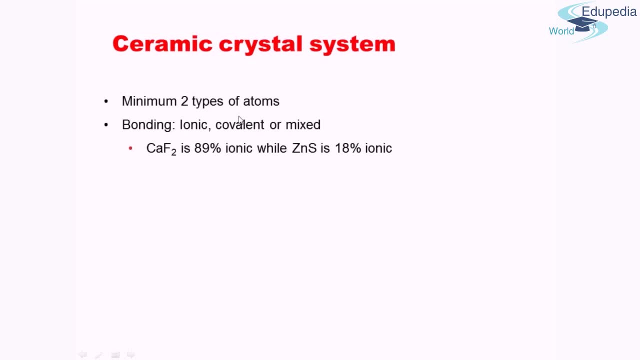 type of atom. there will be a difference in electronegativity between the two kind of atom. they may be quite close in electronegativity. they might be very further away in electronegativity from one to another right and depending on how far, how different is the electronegativity for 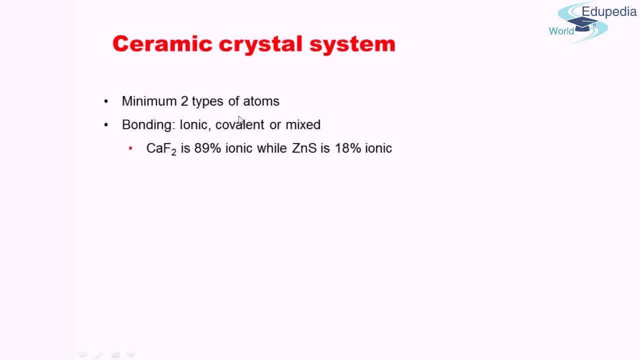 the concerned atoms. the nature of the bonding which will exist between the atoms will be either ionic or covalent, or it can be a mixed intermediate between ionic and covalent nature. right, so when will be the system? when will the bonding be highly ionic? it will be highly. 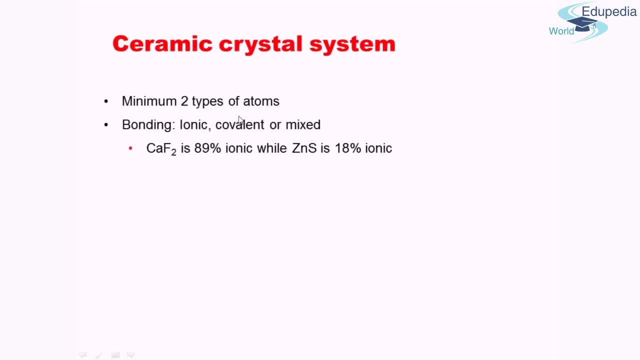 ionic when the electronegativity difference between the two concerned atoms is quite large. on the other extreme, it will be covalent when the electronegativity difference is quite small, obviously, and mixed is for the intermediate cases. now here i have mentioned the 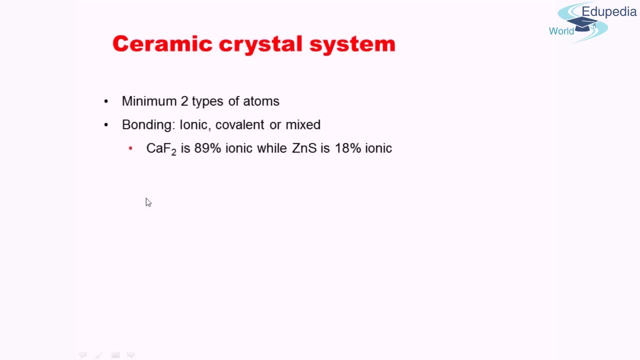 two simple examples which are kind of extreme ends of the spectrum: calcium fluoride, caf2 has 89 percent ionic characteristic, whereas zinc sulfide, or zinc blend, has only 18 percent ionic characteristic, which means that zinc blend or zinc and sulfur, has quite close electronegativity values. 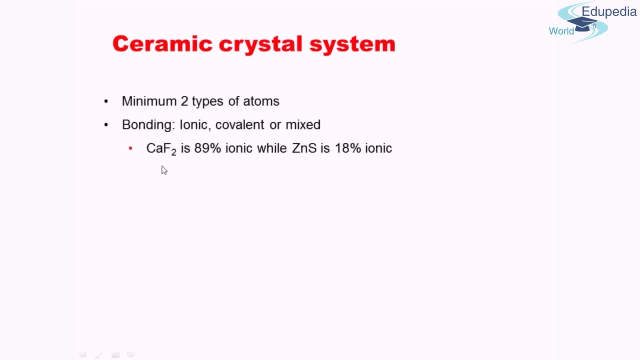 whereas calcium and fluorine are quite far apart in electronegativity. thereby they have ionic nature for the bond formed. right now that we know that it, it can be either ionic or covalent. in case the atoms concerned are of the ionic nature, that is, they are separated with the large 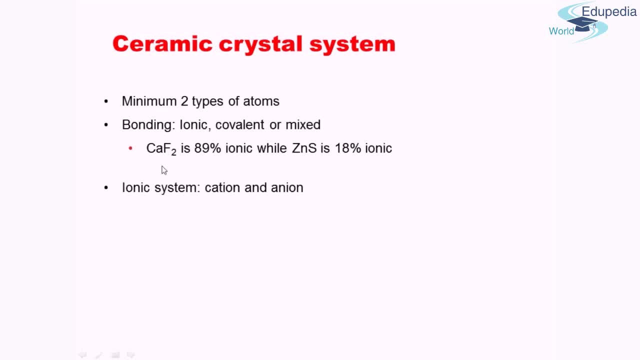 of electron- large difference in electron- then what we can consider is that, instead of considering two different kind of atoms, we can consider them as ions. right, like the one which will be electropathic positive will be acting as the cation, whereas the one which will be 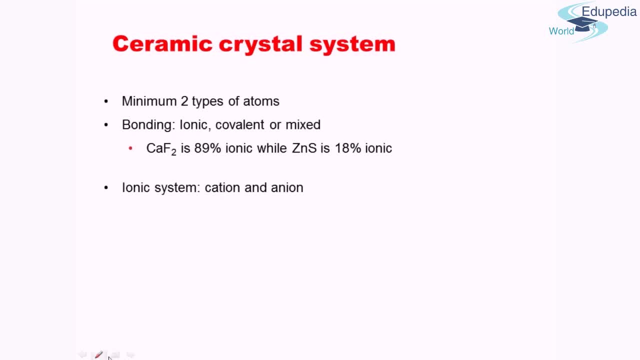 electronegative will act as the anion, for example, in our calcium fluoride case. what I can do is I can take Ca2 plus as the cation and F minus as the anion, right, so this can be translated into an ionic system rather than. 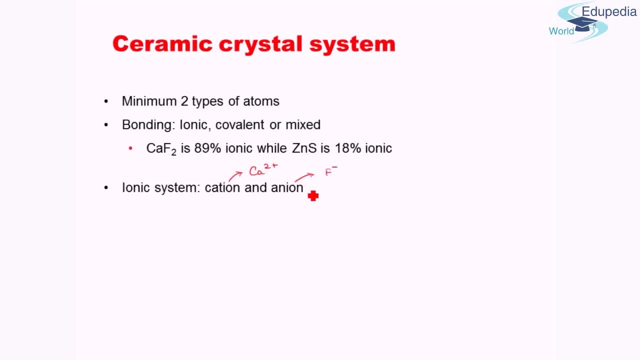 independent atoms, and this helps us visualize the thing that there is a attraction existing between them due to the ionic nature. now that we see that there is a coexistence of cation and anion, this brings into picture the concept of charges. right, obviously, there, cation will have a positive charge, anion. 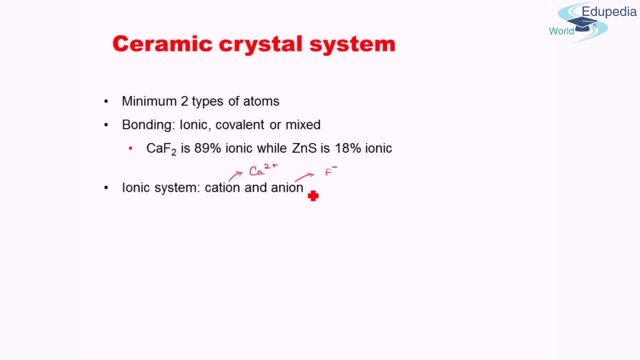 will have a negative charge, but as such, the whole crystal system cannot remain charged. it has to be electrically neutral. therefore, one bottom line or one important criteria for the crystal system to be sustainable is that the charge given by the cation should counteract the charge given by the anion. 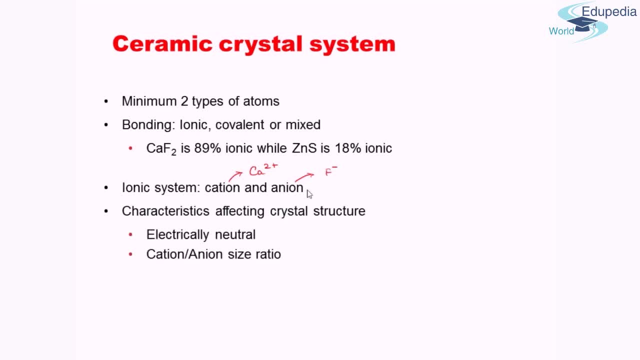 ok, that's what is presented here: characters affecting crystals. specifically. what it means, that is that, depending on that, on what characteristic will the crystal structure affect the anion? please watch from the description so we can say that, whether the cap or the energy will be the same or minus. no, 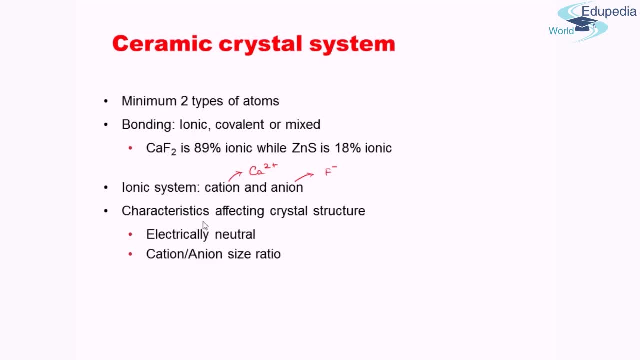 and in согласism the crystal is amputated. so this is necessarily a question of how will the earth still function in the future standard pressure. due to this, there must actually be a vibration that will be generated during the function of the cation system. so there should be a 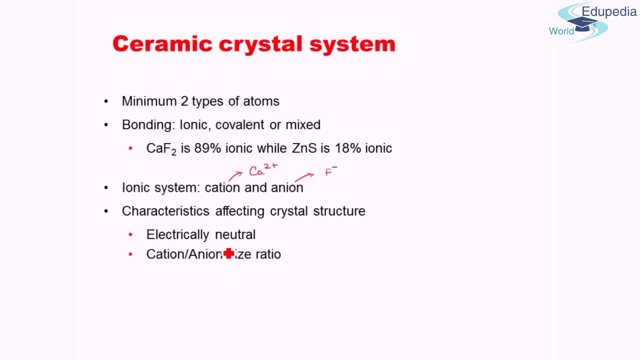 vibration light that will actually be radiated and the efficiency of the ideation just depends on that. is that crystal structure, like the example over here, if we have calcium 2 plus and fluorine 2 minus, what this means is that for charge neutrality to be maintained, there has to be a single calcium 2 plus. 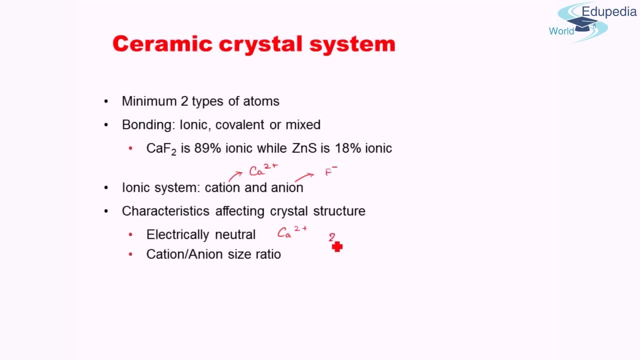 and against each single calcium 2 plus, there has to be 2 fluorine minus. right. there has to be a ratio of 1 is to 2 between calcium and fluorine for the electrical neutrality to be maintained. this is how the crystal structure is being affected by electrical neutrality: the maintenance. 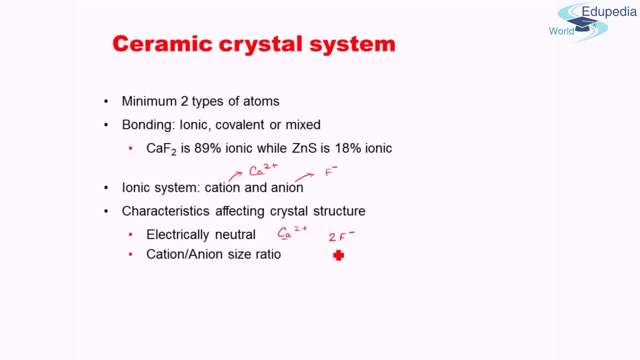 of electrical neutrality, that is, this ratio has to be maintained. similarly, if we take another example, let's say cesium fluoride, CSCL. now here we have CS plus and CL minus. since the charge is only plus and minus, the ratio remains 1 is to 1, whereas here the ratio becomes 1 is to 2. 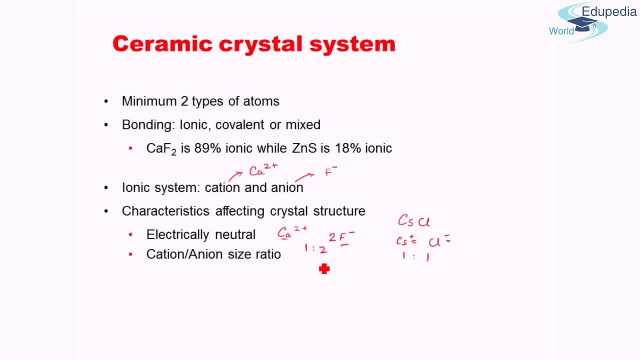 okay, so you get the point which i am trying to make. second, cation to anion size ratio. what do i mean by this? the size of cation. if you come to think about it, cation is formed by losing electrons. anion is formed by gaining electron. right thereby, cation normally will have. 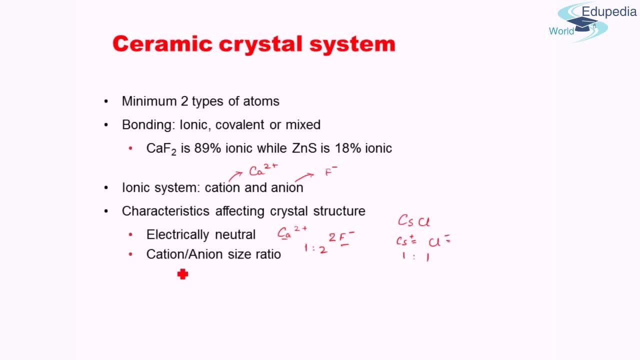 a size smaller than anion because, on losing electron, it loses its outer shell and it its size becomes smaller. anion, on the other hand, does not lose the outer shell, rather it is gaining the electron. thereby it further enhances in size due to further repulsion created between 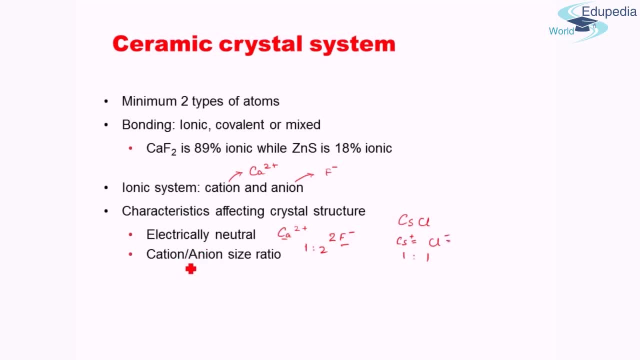 the neutrons. so the cation to anion ratio, size ratio, kind of determines what will be the crystal structure. we will see this in more details in the next slide. there you will get much more clarity about what i'm trying to talk. but point to take home here is that the cation and anion have different sizes and the specific ratio. 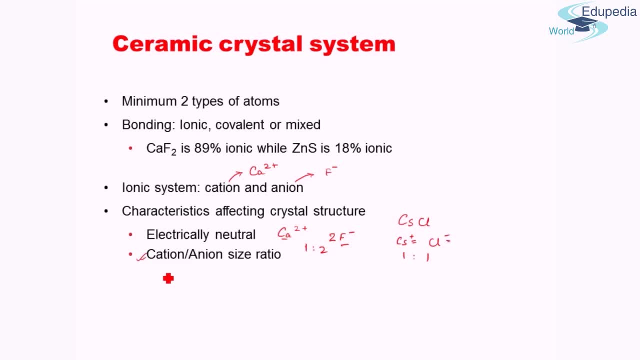 of a given combination will define how the crystal structure will behave. and why is it so? let's see the opposite charges, that is, cation likes to have maximum number of anions surrounding it and anion likes to have maximum number of cations surrounding it. right now, if there is a large 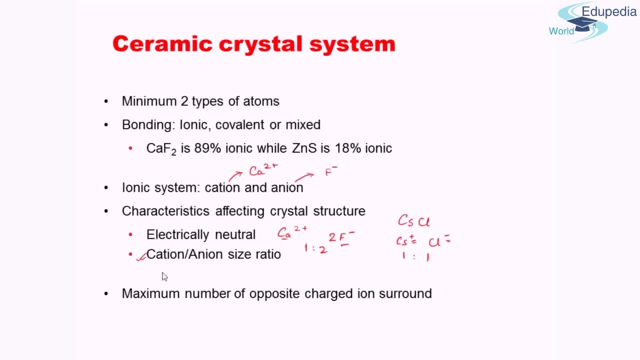 difference in size between the cation and anion. suppose that the cation is very, very small compared to the anion, then it can be difficult to accommodate a lot of anions surrounding the cation, whereas if the cation is of larger size, more number of anions can surround the cation. 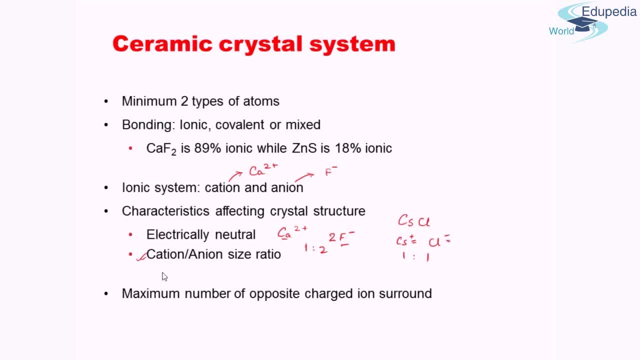 thereby the ratio- size ratio actually affects the crystal structure. also, the coordination number depends on the size ratio. how come? because the coordination number is nothing but the, the how many pieces or different atoms are surrounding a given atom. okay, so more is the size ratio, that is, or let's put it this way, smaller is the cation size, less will be its coordination number. 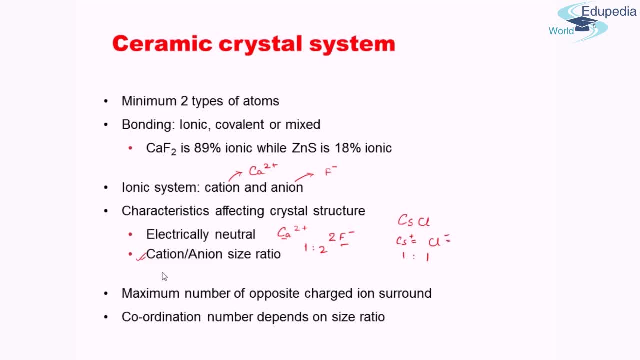 because lesser number of ion anions can surround it, more the cation size, more will be the number of anions surrounding it. thereby more will be the coordination number. okay, so here i have given you a picture about the idea of cation to anion size ratio and how it influences the crystal structure. 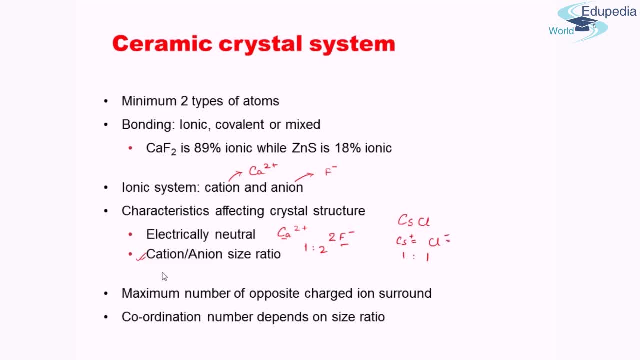 next couple of slides, once we'll talk about what is the stable configuration for cation to anion size ratio under which a ceramic crystal structure can exist and, second, what are the different ranges of cation to anion size ratio and, correspondingly, the different crystal structure. 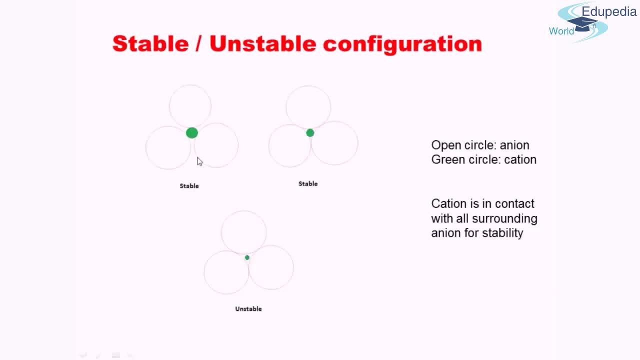 let's see the picture. let's see first for the stability. okay, so here we see three scenarios. i have put three different anions which are hollow circles, and the green circle over here is a cation and, as we can see, cation is smaller than the anion. now for the three different anions in this case. in the first case, 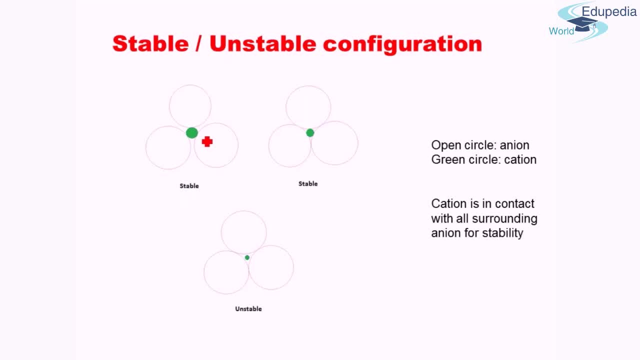 the cation is touching all the three anions. in the second case also, the cation is touching all the three anions, but it is kind of the limiting case. if the cation was even a little smaller then it would not touch all the three simultaneously. 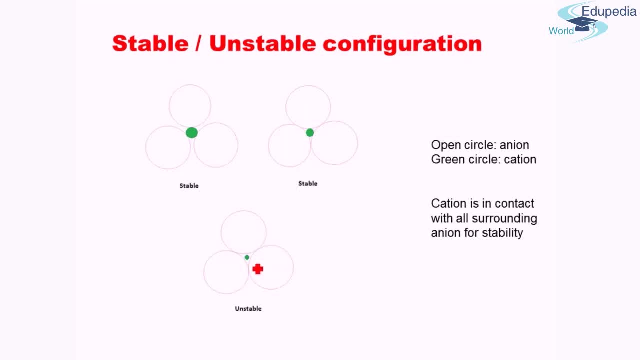 whereas in this case, in the third case, what we see is that the cation is, in fact, smaller than the minimum size which is required for it to touch all the three anions. now you'll say what is so important about this size? the important part is that the cation is not touching all the three institutions. 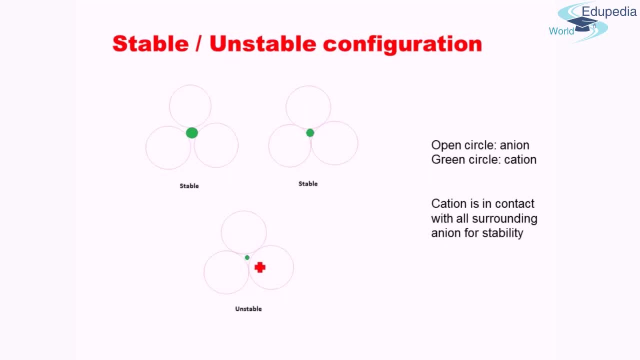 is that, for the stability of the configuration, the cation needs to touch all the atoms surrounded it, surrounding it, or all the anions surrounding it. therefore, this and this structure are stable, and this is the limiting case. this is the limiting, limiting case, whereas this structure is unstable. 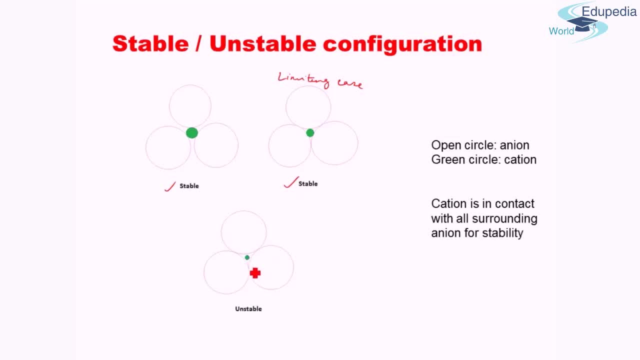 because the cation is not in contact with all the surrounding anions. it may be in contact with this two, right, if this was somewhere here, then it this cation would have been contacted with this and this, but it still would not have been in contact with the third one, thereby this, this. 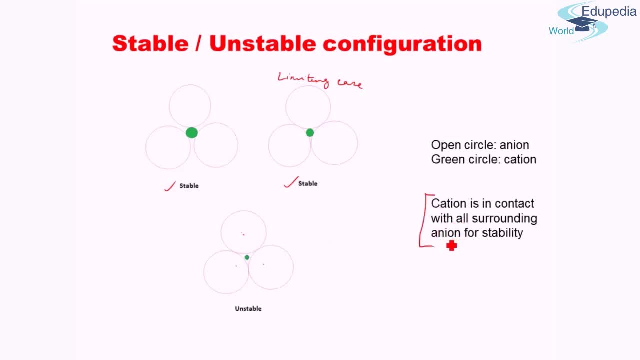 contract that the cations should be in contact with all the surrounding anions would not be valid in this case. so this is the fundamental unification. this is the reason why we need to remember this: for stability, the cations should be in contact with all the surrounding anions. 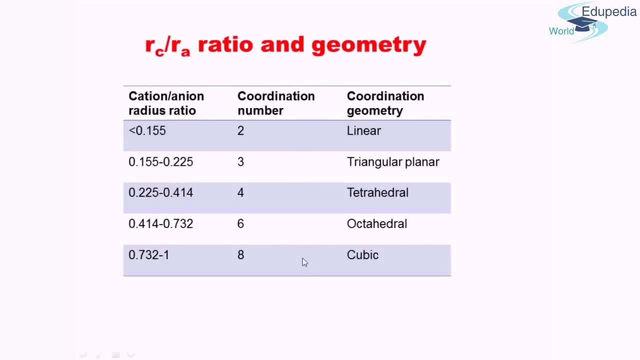 okay, now let's see the size ratio which i was talking about: rc by ra. this is the radius of cation and this is the radius of anion and its relation with the geometry. so, as i said that the cation should be in contact with all the surrounding anions and this is the radius of anion. 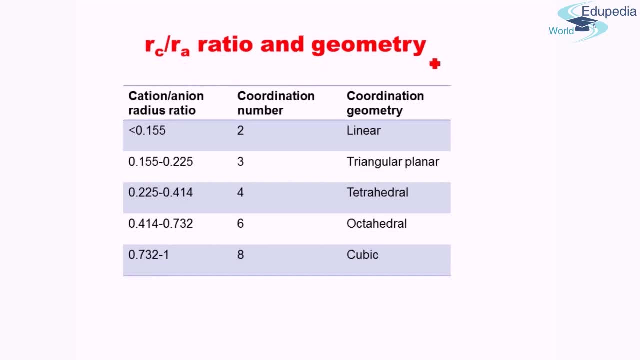 normally the cation will be smaller than the anion. Therefore, Rc upon Ra will normally be less than 1.. Okay, So let us see the different cases for Rc by Ra less than 1.. And, mind you, this coordination number which we have generated here for different cation to anion ratio and the 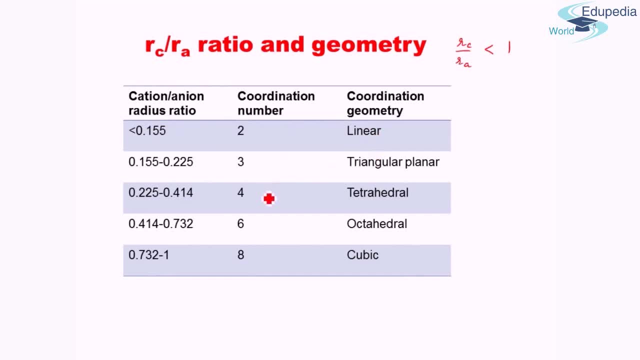 corresponding coordination geometry. all this can be mathematically derived using geometry. This is: this has nothing to do with metallurgy or material science. This is basic geometrical calculations, but I will not go into details. I will give you the output of the different ratios. 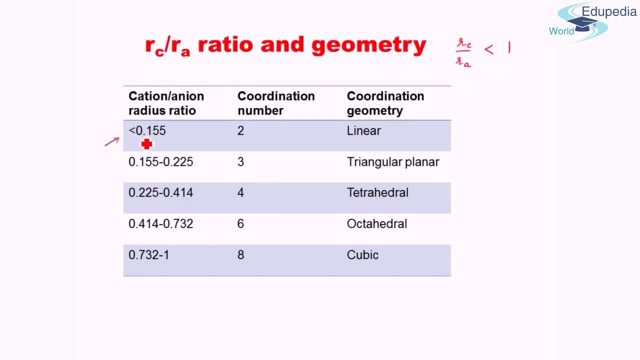 The ratio. if the ratio of cation to anion is less than 0.155,, then what we will have is a coordination number of 2 and the coordination geometry will be linear. Let me show how it will be. What will happen is the anion will be two small particles, Okay, And the cation, as I said. 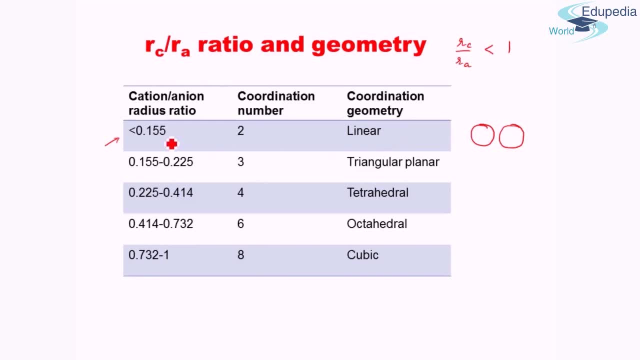 is less than 0.155 times the radius of the anion, So the cation will be basically very small, very small, something like this: Okay, And it is touching the first and the second, both anions, And this configuration is linear. 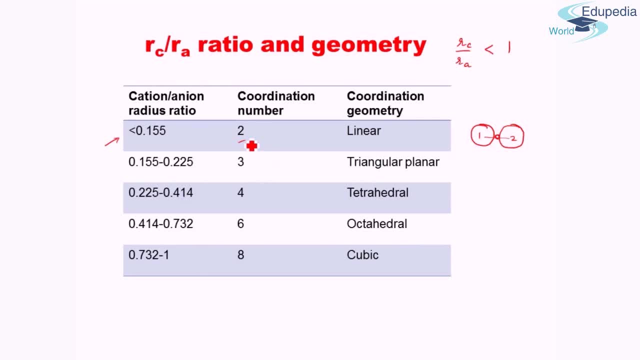 It is a linear pattern, So the coordination number is 2 and the coordination geometry is linear. Okay, The second configuration will be when the cation to anion ratio is between 0.155 and 0.225.. Then the coordination number will be 3.. 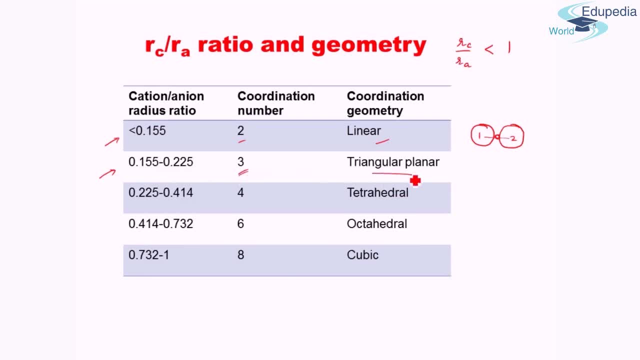 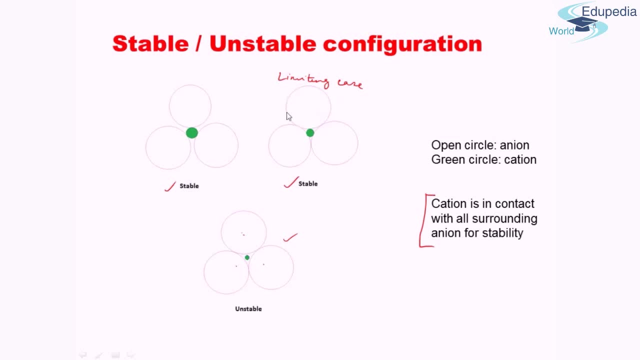 And the geometry will be 0.255.. Then the geometry will be triangular planar. Triangular planar with coordination. number 3 is the same as this one. Here you see that there are three anions And this is my cation, which is lying exactly at the center. 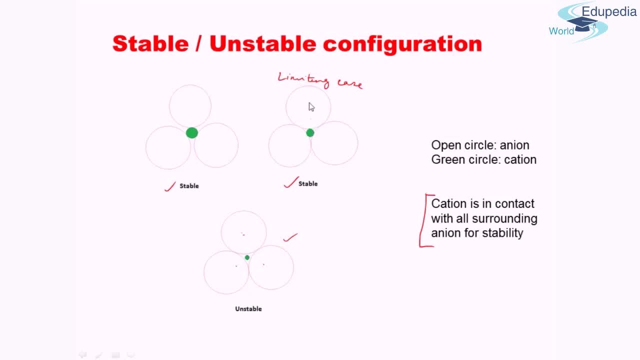 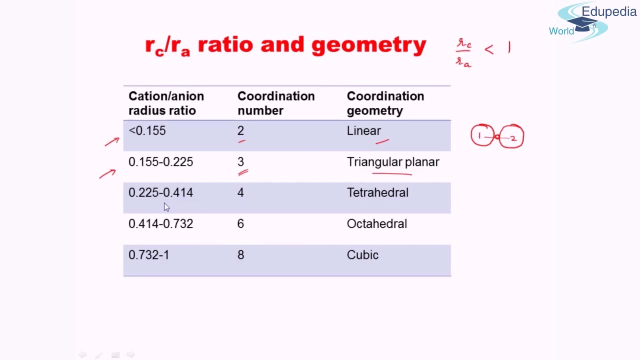 So it is touching three anions And its geometry, as you can see, is in the plane of the paper Right, This is the plane of the paper And it is triangular, So it is called triangular planar. Okay, If the ratio is between ratio of cation radius to anion radius is between 0.225 to 0.0414,. 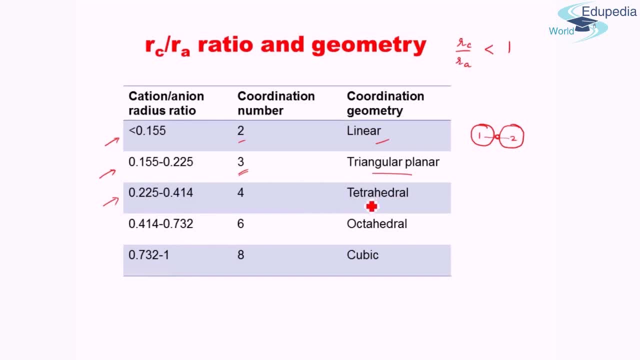 then what we'll have is known as tetrahedral scenario. Okay, Now what is tetrahedral scenario? In tetrahedral scenario, what you'll have? this no longer remains a 2D configuration. This now becomes a 3D configuration. 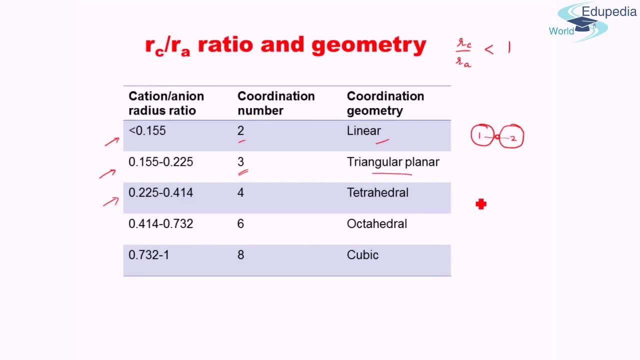 So I'll try to give an idea how this will look, But it might not turn out to be very good representation. Okay, So these three atoms will kind of lie in one single plane. This is my cation. Okay, These are the anions And a fourth. 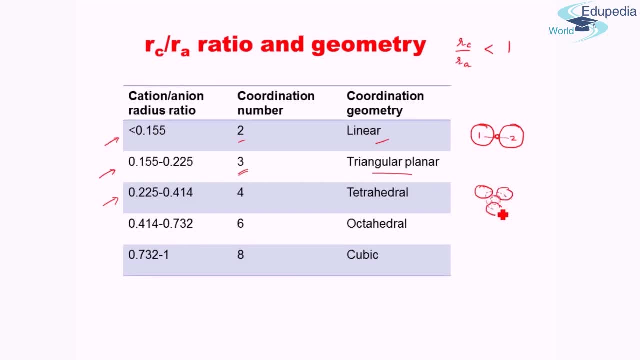 anion will be lying on top here, That is, it is in outside the plane of the paper. Right, These three are in the plane of the paper And this- both the anion and the cation- are outside the plane of the paper. Alternatively, you can think of it something like this, Something like: 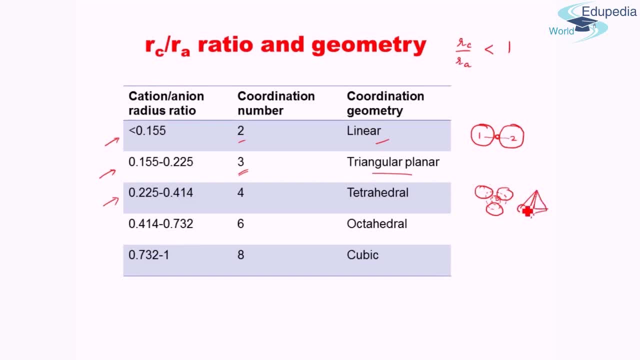 this. So one atom, one anion is here, One anion is here, One anion is here, And fourth anion is here. And there is this anion will be touching each other. Obviously, I cannot show you here. 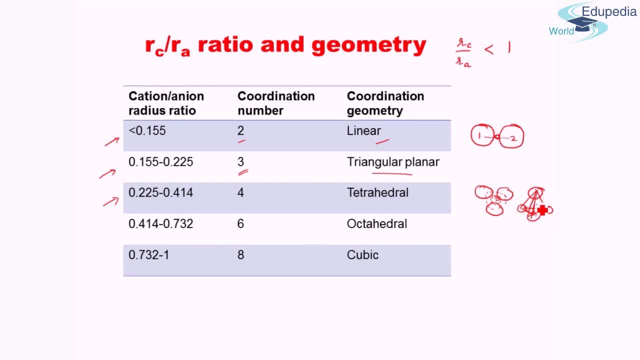 But they will be large enough to touching each other, And in between there will be a gap here which will be known as the tetrahedral void, And in that tetrahedral void will have the cation placed. Okay, So this is, as you can see, a 3D configuration. 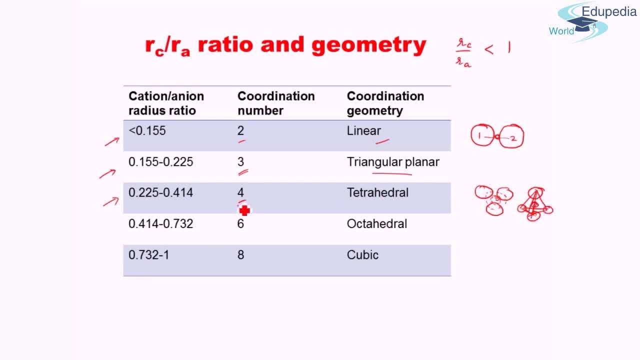 And this we have four coordination number, Because this atom, this cation, will have four atoms surrounding it: One, two, three, four, And the geometry is called tetrahedral geometry. Okay, Now, if the radius ratio between the cation and the anion is between 0.414 and 0.714,, 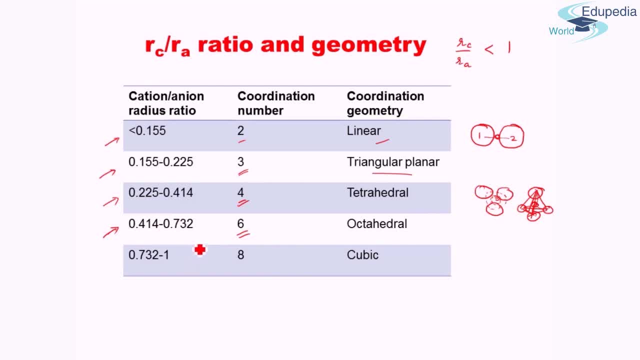 then the tetrahedral void will have the cation placed. Okay, So this is, as you can see, a 3D configuration here, And what we will have is, as you can see, a tetrahedral geometry, Which means that the cation will be surrounded by six anions. Now, how will this look like? 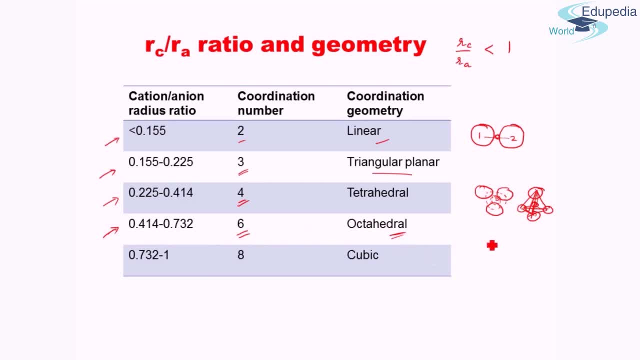 How will the tetrahedral void look like? So what will happen is in the plane of the paper, we will have like four atoms, right, Four anions. then one anion will be within the plane of the vapor. it is inside, it is not in this plane, it is. 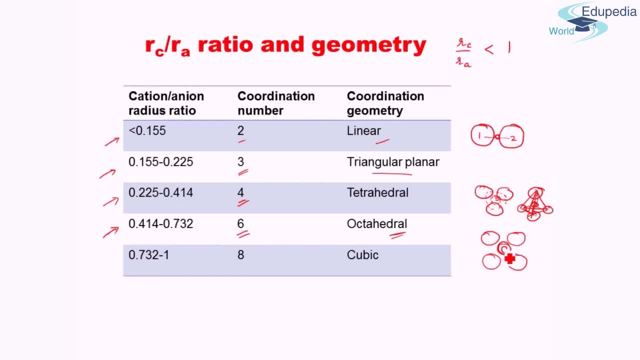 inside and over here will be my anion, rather cation, placed. so this one, two, three, four, four anions- this is the fifth anion inside the plane of the vapor, this is my cation, and there will be a sixth anion on top of the plane of the vapor. so, basically, what we are seeing here is something. 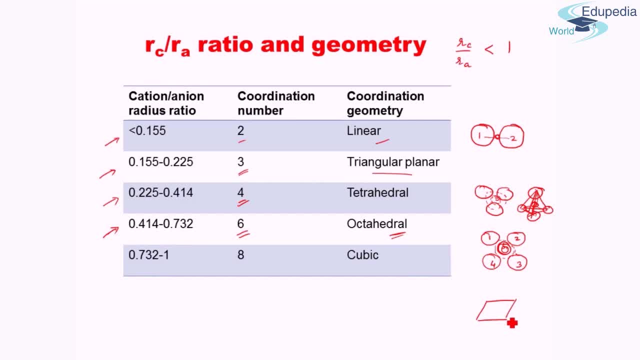 like this, something like this. okay, so one, two, three, four. this four are the. this four anions at the plane of the vapor. one anion will be at below the plane of the vapor, one anion will be. this passes through the center, at the top of the plane of the vapor. 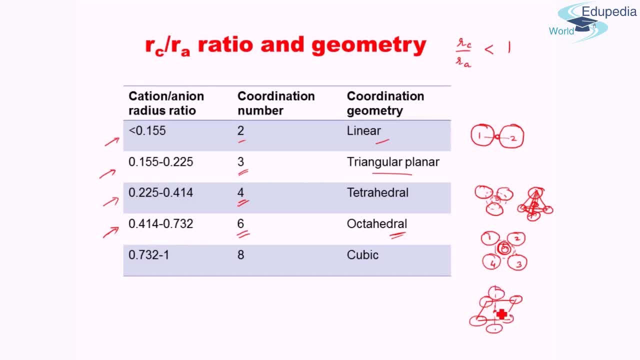 and bit between over here, there will be a void. this will be filled by the cation. so now what will happen is- and this cation will be touching all the six anions, so we have one, two, three, four, five and six, six coordination number, and this is known as my octahedral geometry. okay, why octahedral? because 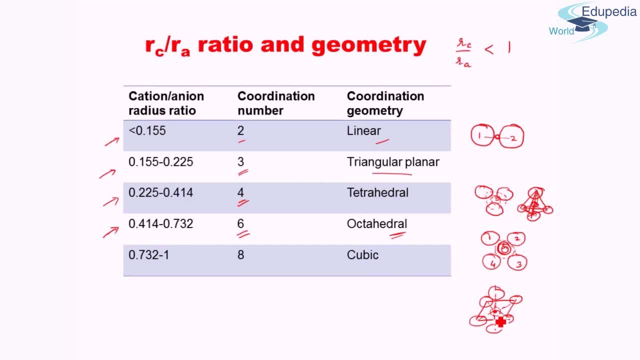 it sounds like there are six atoms surrounding it, but octa means eight. so the reason is, if you kind of draw the structure like this, so one phase, two phase, three phase, four phase and similarly four phases at the bottom, so there are eight phases within which the cation is confined inside. 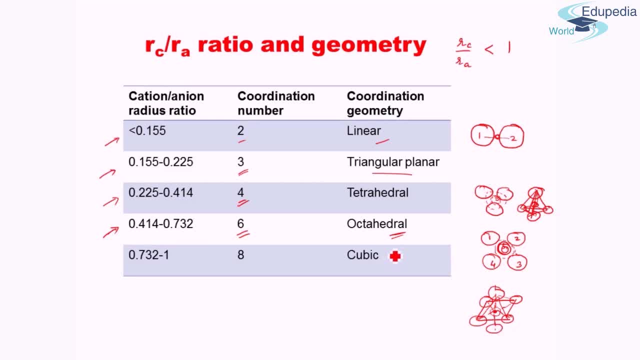 okay, so now you have got idea about what is the octahedral geometry. finally, if the radius ratio between the cation and anion lies between 0.732 and 1, then we will have what is known as the cubic geometry. you and the coordination number will be eight and, as you can think, with the name cubic, what will? 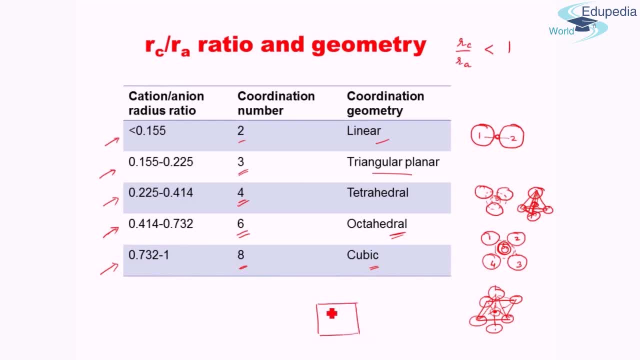 happen similar to our crystal structure for the metals or for element metal elements. what will happen is that the anions will be at the eight corners right- one, two, three, four, five, six, seven, eight- and there will be a void over here inside and that void will be filled by the cation and this void is